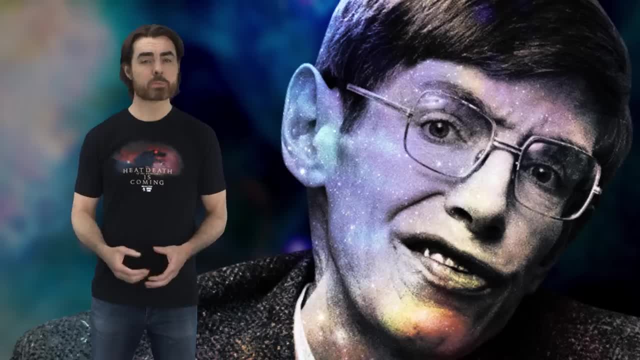 He was perhaps the greatest genius of our time. Stephen Hawking peered behind the curtain of reality and glimpsed the true workings of the universe. He inspired all of us to pursue our curiosity no matter the obstacles. However, his true legacy is his work He made profound. 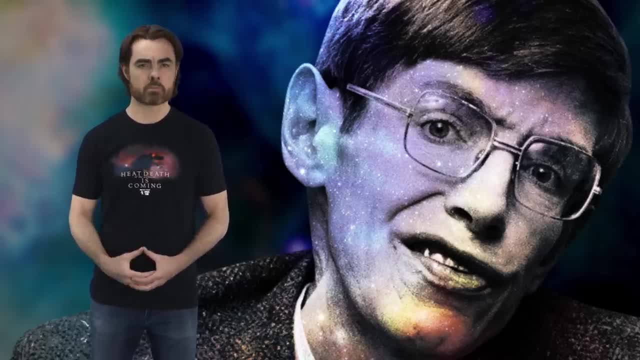 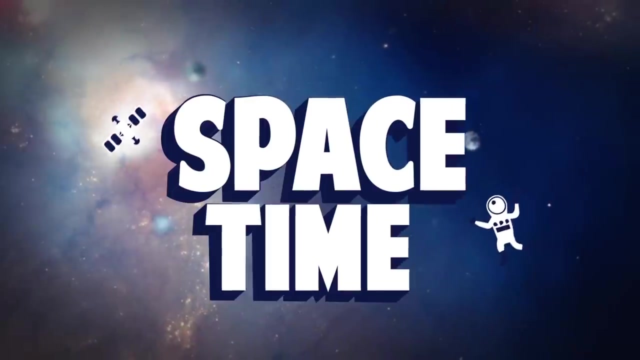 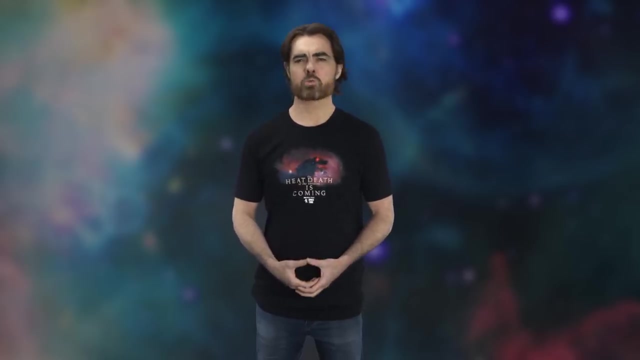 contributions across physics, from quantum theory to cosmology. Our tribute is to bring you Stephen Hawking's most famous discovery. I'm Matt O'Dowd. This is Space Time and it's time for Hawking: Radiation. Soon after Einstein revealed his great general theory of relativity in 1915, physicists realized: 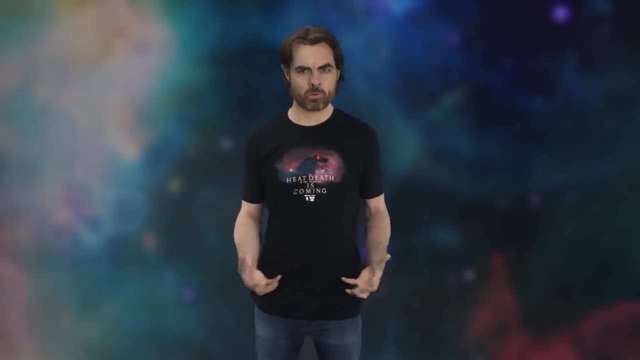 that it allowed for the possibility of catastrophic gravitational collapse in places of extreme density, like the dead core of a massive star. Space and time could be done together. They dragged inwards to create a hole in the universe, a boundary in space-time called an event horizon that could be entered but from beyond which nothing could return Once. 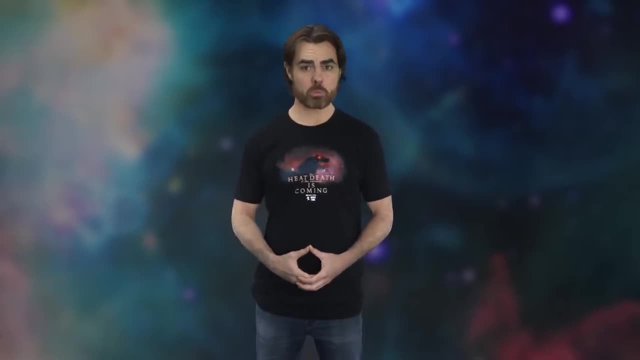 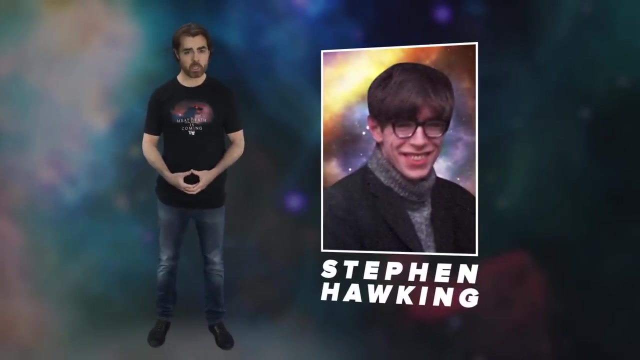 formed, there was nothing in theory or imagination that could bring material consumed back to the outside universe. These black holes should exist forever, only growing, never shrinking, Or so we thought until 1974, when a young physicist named Stephen Hawking came to the. 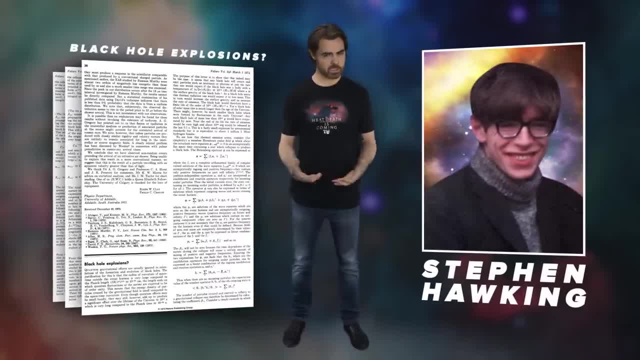 table and published a paper in Nature entitled Black Hole Explosions. In this and in a follow-up 1975 paper he attempted a new union of quantum mechanics and general relativity to show that black holes should not be so black. after all, They should leak, They should emit what? 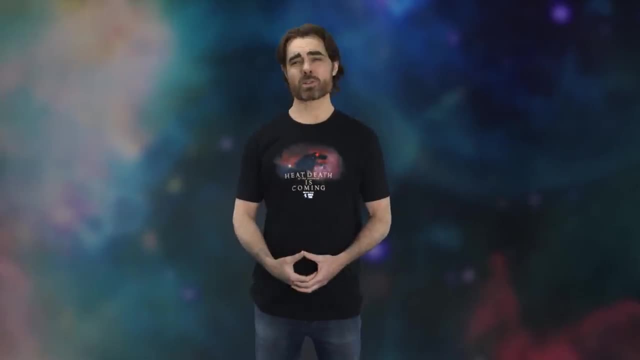 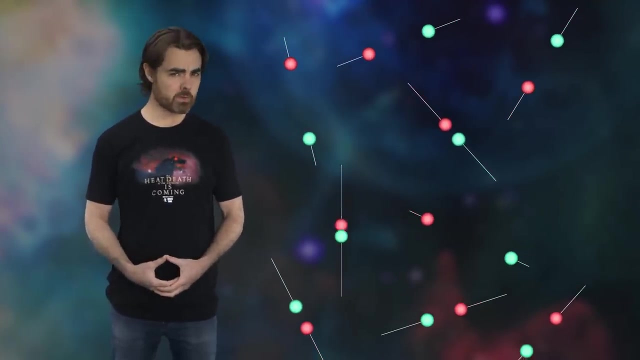 we now know as Hawking radiation. There's a popular description of how Hawking radiation works. It goes something like this. It goes something like this: Empty space seethes with activity, as pairs of virtual particles- matter and antimatter- spontaneously appear. 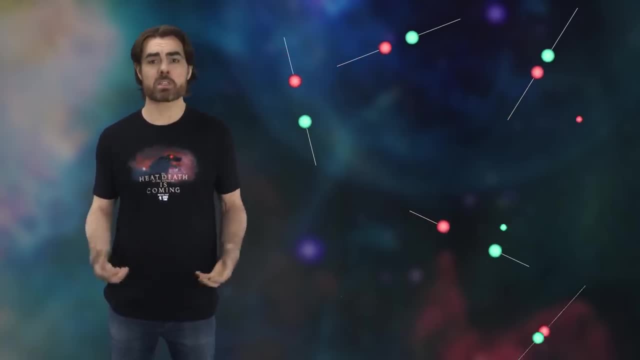 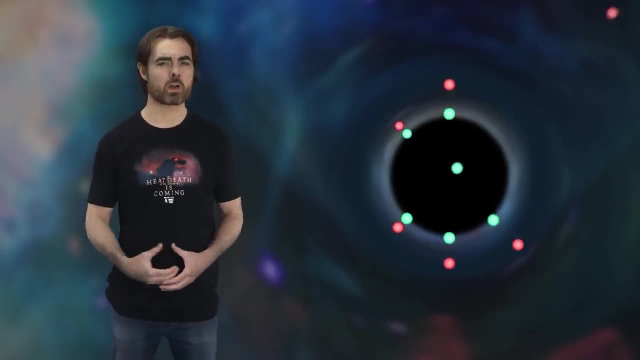 and then annihilate each other briefly, borrowing energy from the vacuum itself. But when this happens near a black hole, sometimes one of the pair will be swallowed by the event horizon, leaving the other free to escape and taking its stolen energy with it. 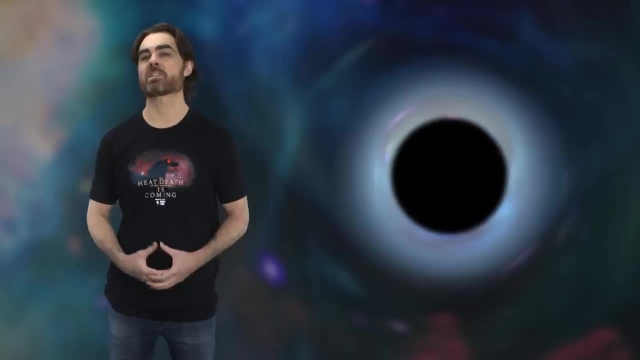 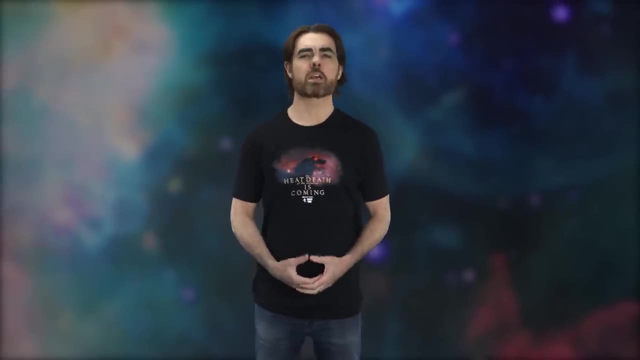 That energy can't come from nothing, and so the black hole itself pays the debt by slowly leaking away its mass. This is a nice picture, but how accurate is it? In fact? if we follow the narrative of Hawking's original calculation, the story sounds rather different. 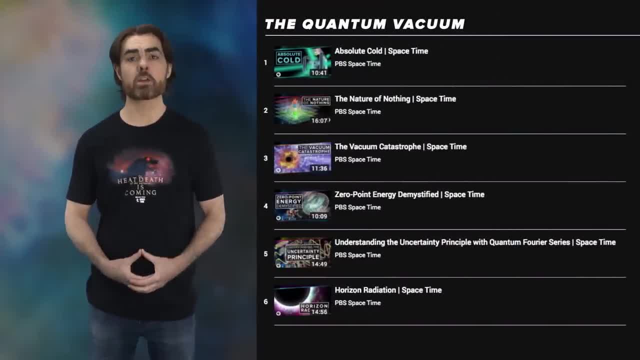 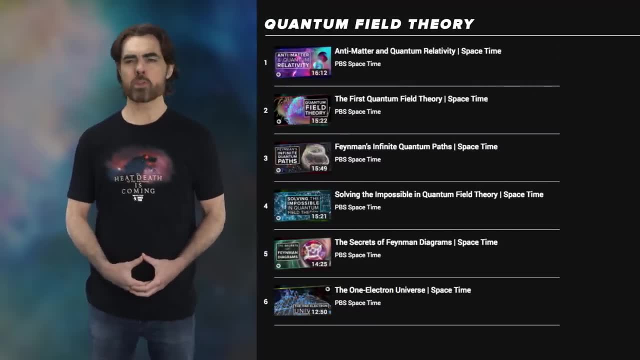 We've come a long way over the past few months, building up the knowledge we'll need to follow that calculation. Rewatching some of those episodes either now or after this video will be helpful, But if you think you're ready, let's take a deep dive. 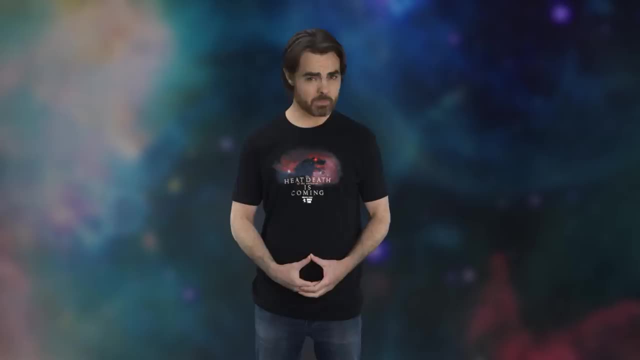 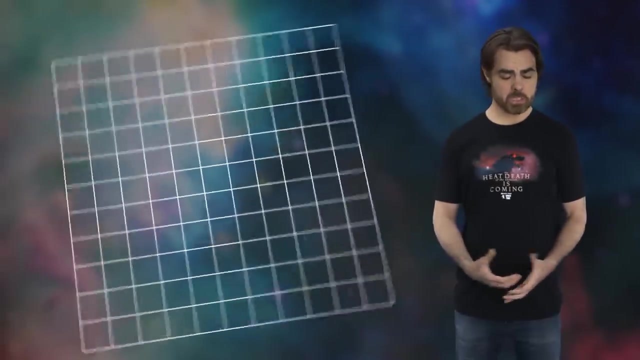 into the quantum field theory of curved spacetime to glimpse the true nature of Hawking radiation. Actually, a quick QFT refresher can't hurt. Space is filled With quantum fields. they can oscillate with different frequencies, much like the many 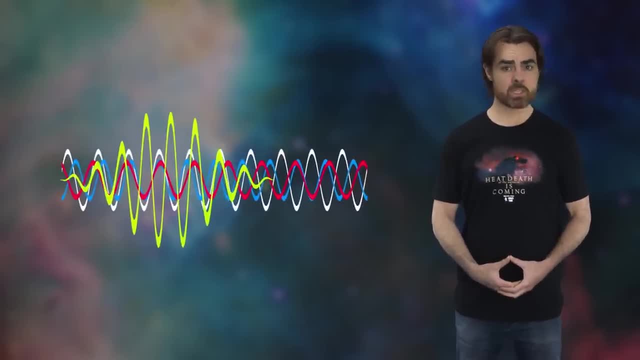 possible vibrational modes. on a guitar string, A particle is like a note on the string And just like a real guitar note. real particles tend to be comprised of many vibrational modes. Those underlying vibrational modes are still present in the absence of real particles. 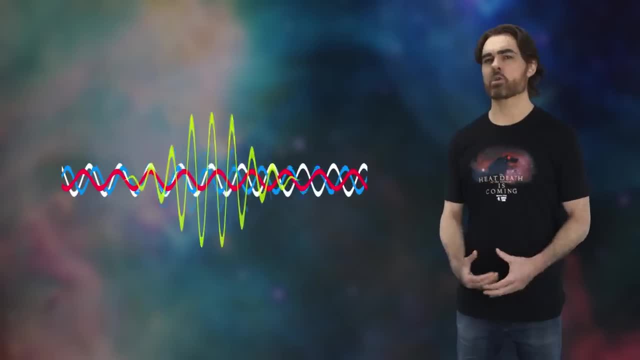 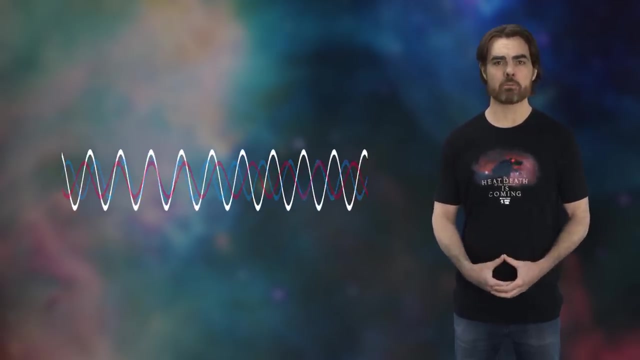 They fluctuate in energy due to quantum uncertainty, and those fluctuations give us what we think of as virtual particles. Now, don't take the existence of virtual particles too seriously. They're really just a tool for calculating the infinite ways in which a fluctuating quantum field can behave. 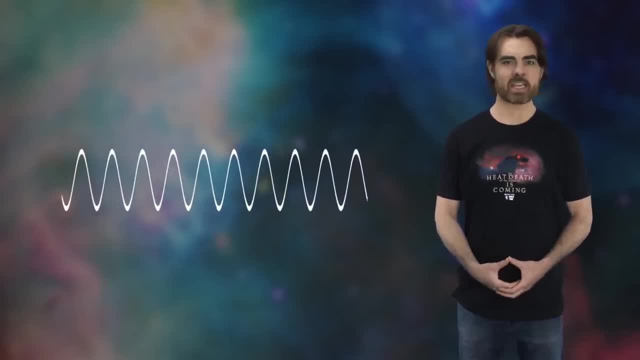 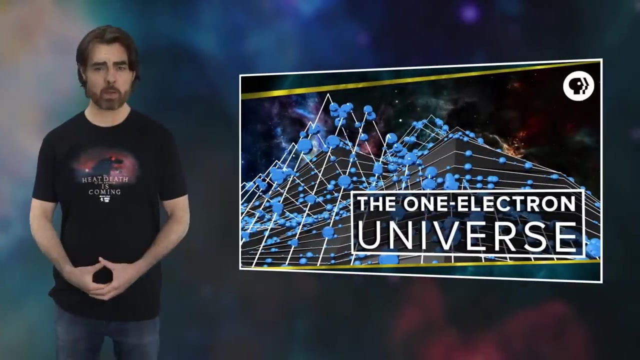 One way that quantum fields are very different to guitar strings is that they can have both positive and negative frequencies. A negative frequency can be thought of as a mode that travels backwards in time and can be interpreted as corresponding to antimatter. Now, that's a whole level of weird all on its own. 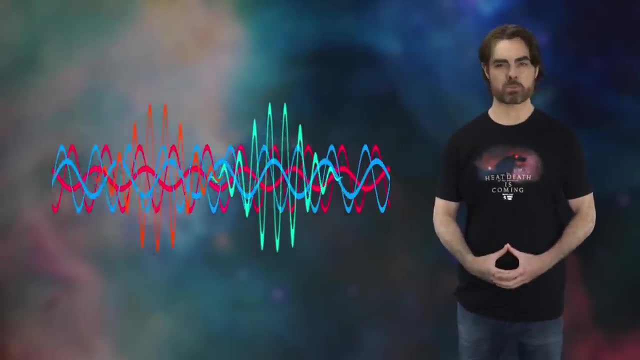 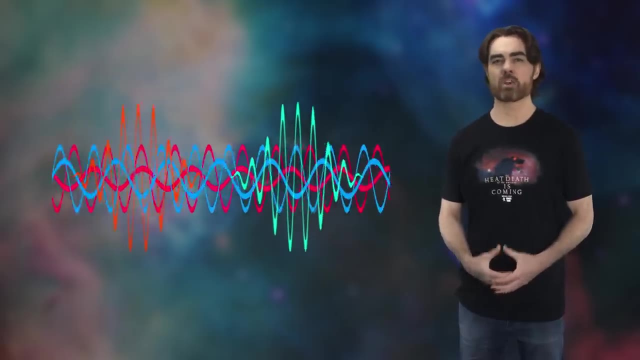 and we talk about it here. When a quantum field is in a vacuum state, there's a balance between positive and negative frequency modes, which you can crudely think of as a balance between virtual matter and antimatter particles. These all virtually annihilate or cancel out. 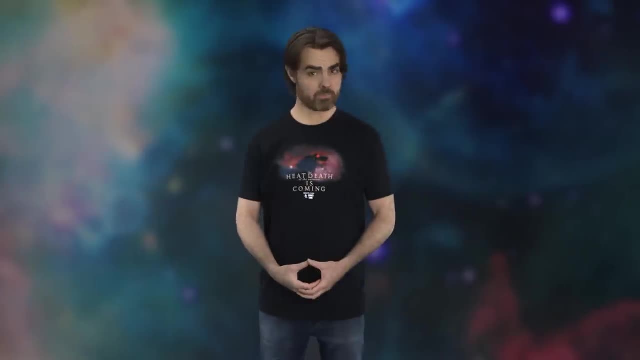 so that no real particles exist. This is all fine in flat space, but spatial curvature can mess with the balance of the underlying quantum field modes by introducing horizons. Horizons cut off access to certain modes of the quantum fields, disturbing the balance that 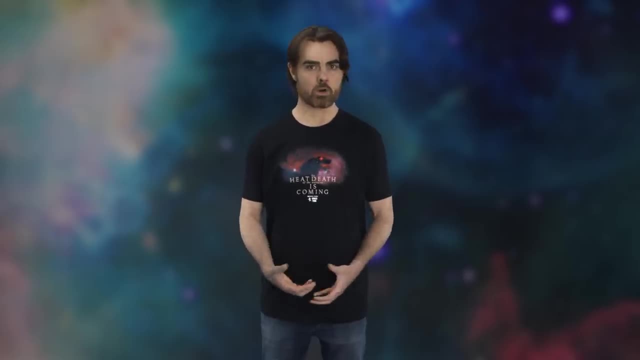 defines the vacuum. Stephen Hawking knew that black holes, with their insane spacetime curvature, would wreak havoc on quantum fields in their vicinity. But what would the effect be? To answer that properly, he would need a full union of general relativity and quantum. 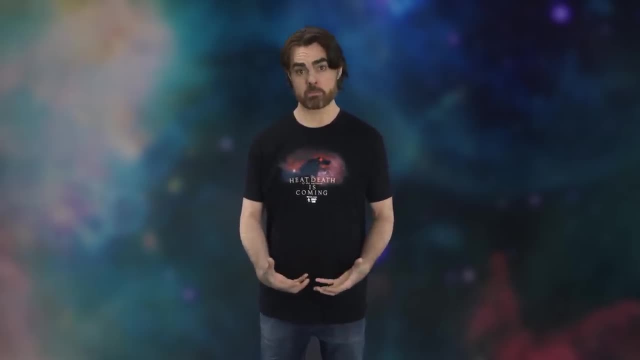 mechanics, a theory of quantum gravity, a theory of everything. It didn't exist then, and it doesn't exist yet. Not to be deterred by the impossible, Hawking came up with an ingenious workaround: The narrative of Hawking's mathematics. 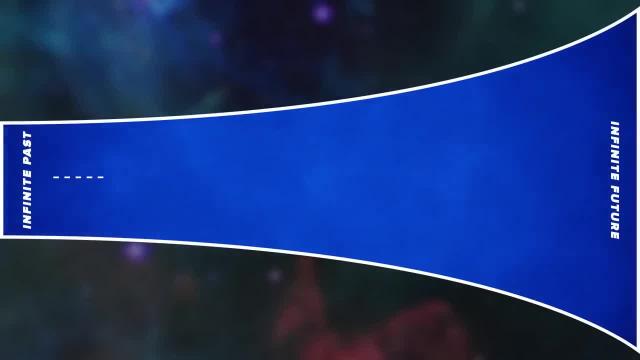 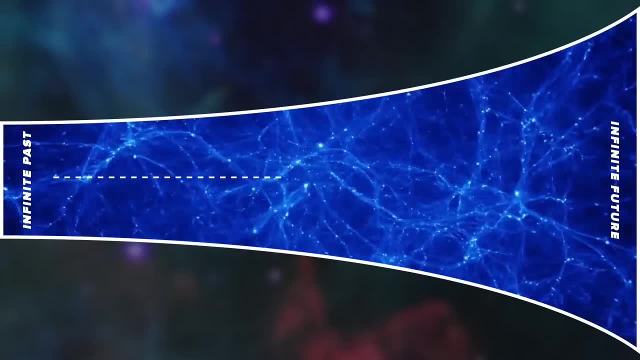 goes something like this. He imagined a single spacetime path, a light speed trajectory called a null geodesic. It extends from far in the past to far in the future. This is a perilous path. It passes through the location of a black hole. 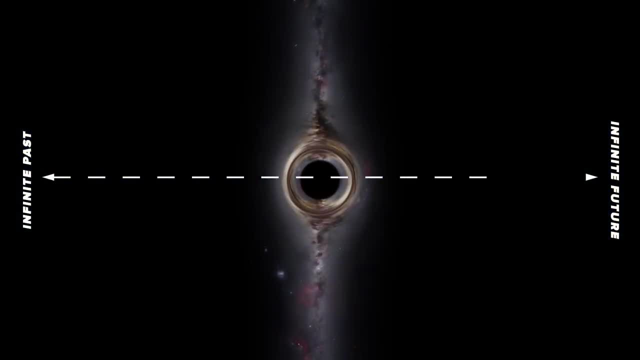 in the instant before it forms. In fact, it is the very last trajectory to do so. It emerges barely ahead of the forming event horizon. Hawking imagined a simple quantum field tracing this path, a field that is in a perfect vacuum state. 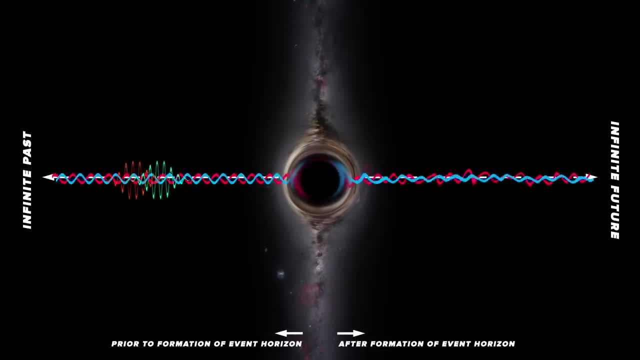 before the formation of the black hole. But he found that the close shave with the black hole disturbs the fundamental vibrational modes that define the fluctuations of the vacuum. By the time this trajectory has found its way back out into flat space again, those fluctuations, 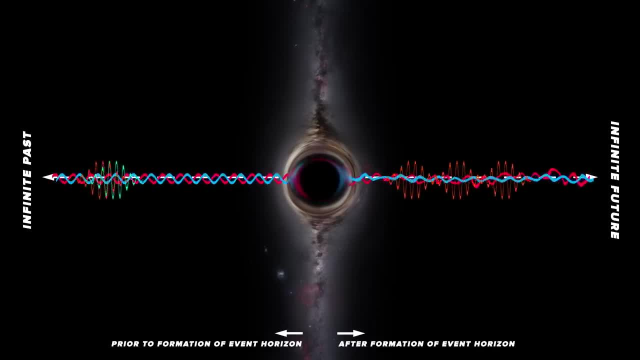 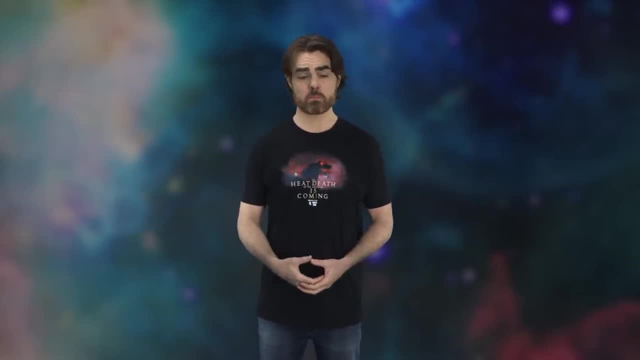 look like real particles. A distant future observer sees radiation coming from the black hole. Hawking's imaginary path from the distant past to the distant future- It was brilliant. It allowed him to compare the state of the vacuum in two regions of flat space. 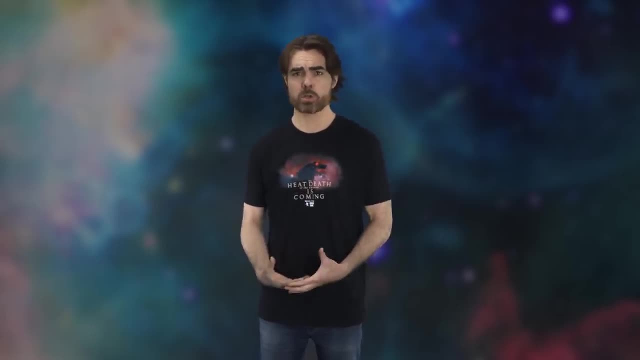 far from the black hole regions where the nature of vacuums, quantum fields and particles are perfectly well understood. But to understand the effect of the close encounter with the black hole, he required an uneasy marriage of quantum mechanics and general relativity. 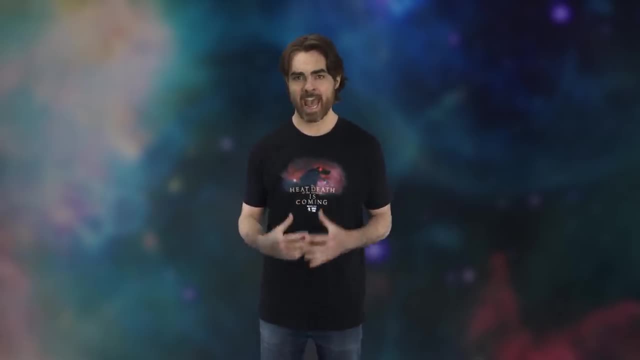 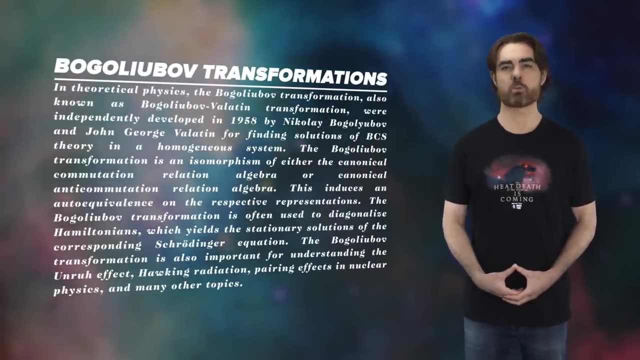 In the absence of a theory of quantum gravity, Hawking needed a hack. That hack was the Bogolyubov transformations. Say that three times Fast. These can be used to approximate the effect of curved space time on quantum fields by smoothly connecting. 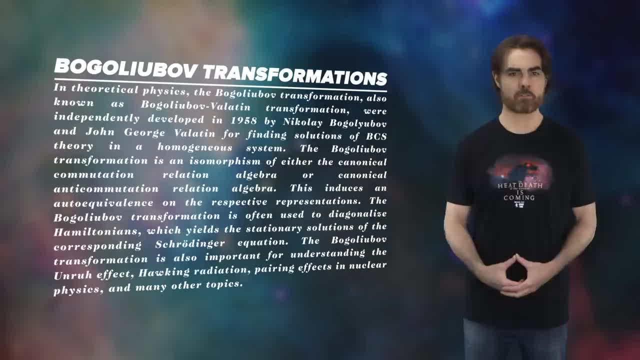 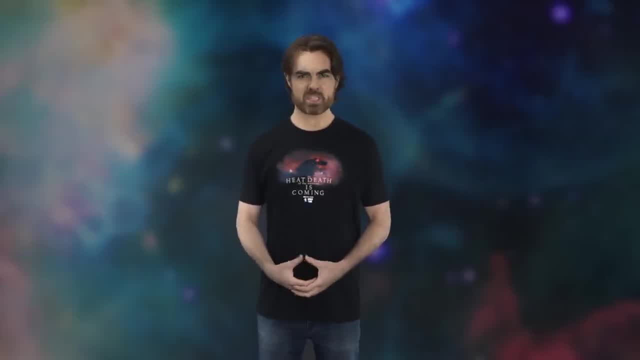 regions of flat space. They describe a sort of mixing of the positive and negative frequency vibrational modes that are caused by that curved space. The physical interpretation of this mixing via the Bogolyubov transformations is tricky. In fact there isn't just one valid interpretation. 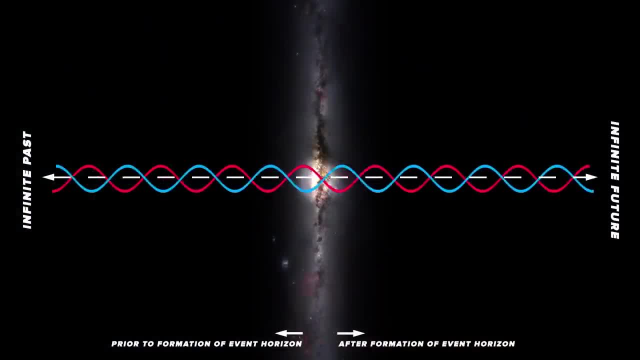 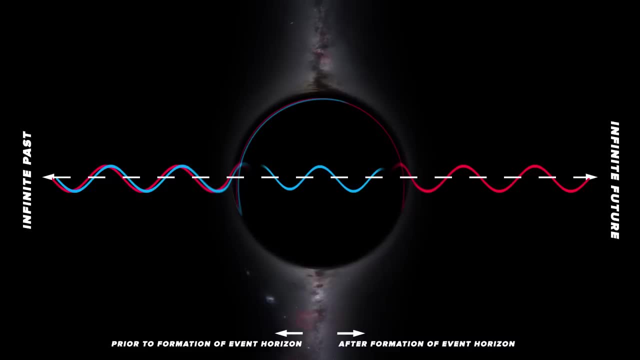 Hawking's calculation talks about scattering. Certain modes of the quantum field are scattered or deflected by the gravitational field of the forming black hole. They are nudged off their narrow escape path and so are lost behind the forming event horizon. Meanwhile, other modes avoid scattering and continue. 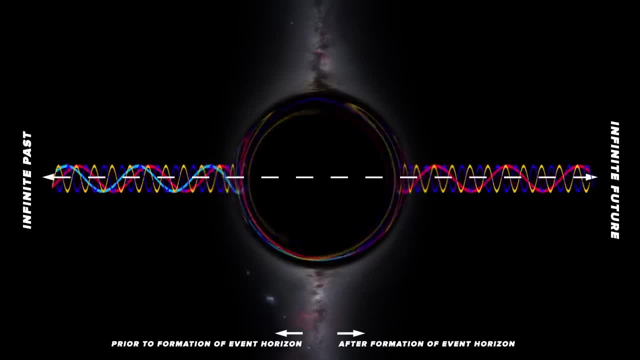 unscathed. With the loss of certain fundamental modes, the vacuum state must be constructed from the remaining modes. That distorted vacuum looks like it's full of particles. The nature of the lost modes tells us what Hawking radiation should look like. Black holes tend to scatter modes with wavelengths similar. 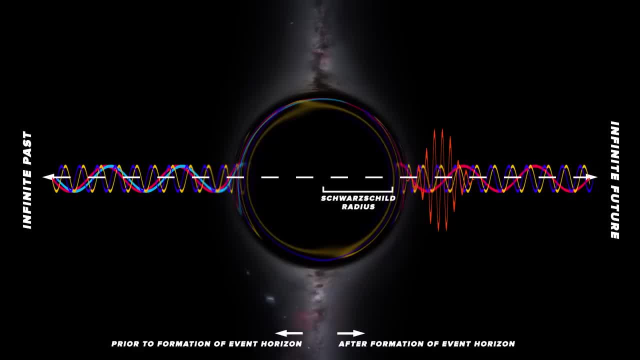 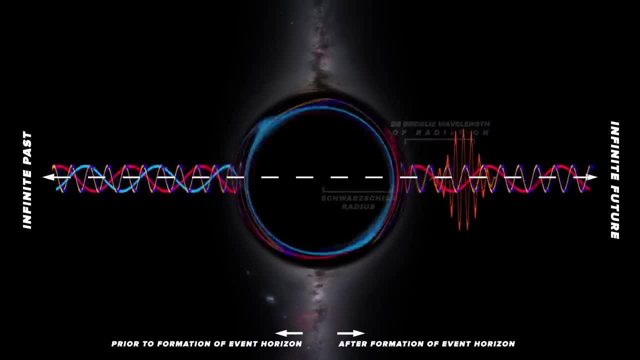 to their own sizes. The quantum field that emerges is distorted in the same wavelength range, and so it produces wave packets. It produces particles that also have wavelengths about as large as the event horizon. So the more massive the black hole, the longer the wavelength of its radiation. 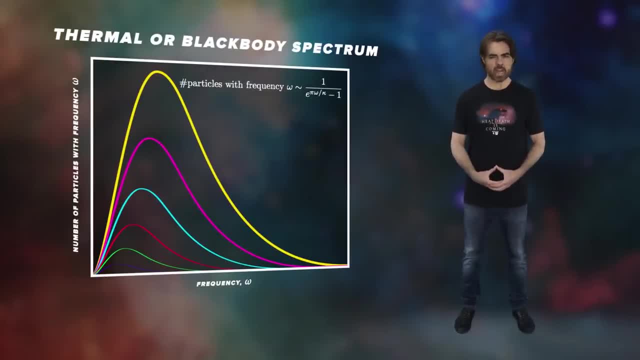 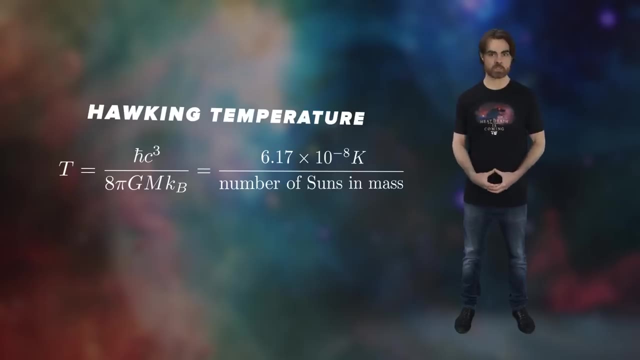 Hawking calculated the frequency distribution of this radiation and found something incredible. It should look exactly like thermal radiation. Black holes should have a heat glow with an apparent temperature that depends on their mass. More directly, it's proportional to the surface area of the event horizon. 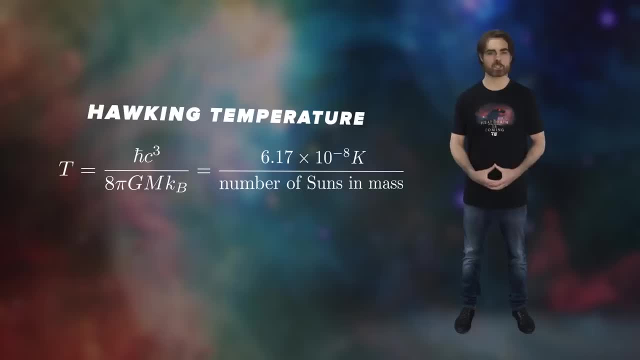 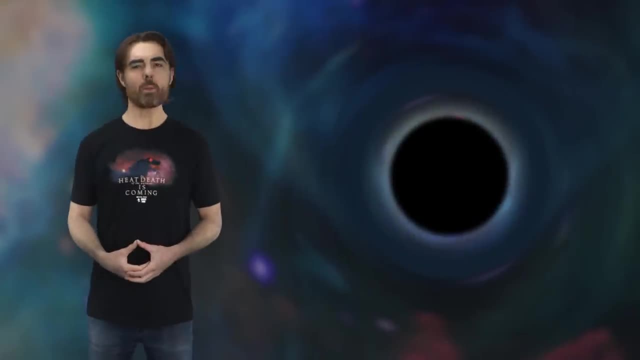 Large black holes should appear cold, radiating excruciatingly slowly, But small black holes should appear hot and the smallest should radiate explosively. OK, so what about the whole picture of particle-antiparticle pairs being pulled apart by the event horizon? 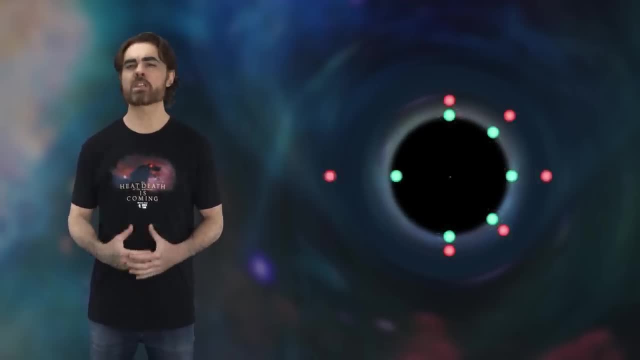 So Hawking's math describes splitting or mixing of these pure positive and negative frequency modes. It's fair to interpret this. We can interpret particle-antiparticle mixing as the promotion of what were once virtual particles into reality And for the escaping modes there. 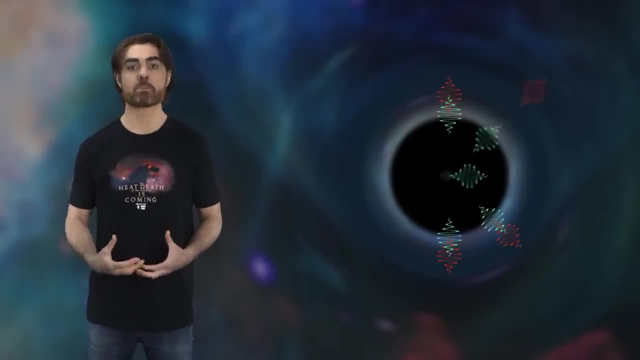 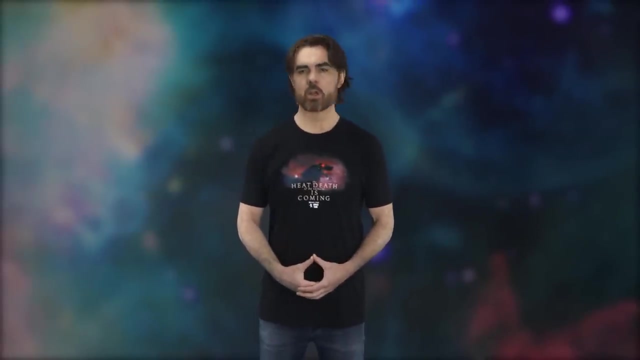 exists a corresponding set of modes linked by quantum entanglement that are trapped behind the event horizon. We can interpret those as corresponding to the swallowed antiparticle partner. So the split matter-antimatter part of the picture is reasonable. But there are reasons to dismiss aspects of this picture. 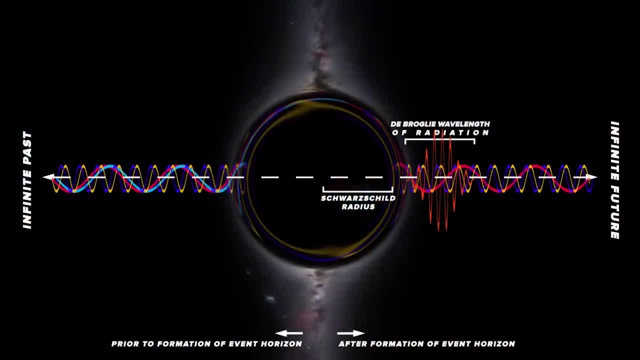 Firstly, this radiation is not localized. Remember that Hawking radiation has wavelengths the size of the event horizon, the size of the entire black hole. Well, these are the de Broglie wavelengths of created particles And they tell us that there is an enormous quantum uncertainty. 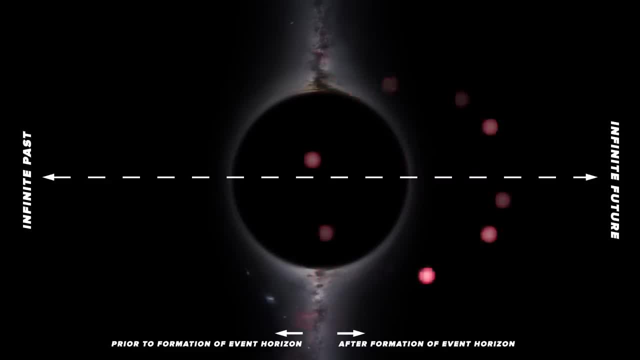 in the location of these particles. Hawking radiation must appear to come from the global black hole, not from specific points on the event horizon. In fact, an observer in free fall through the horizon sees nothing To them. space is locally flat. 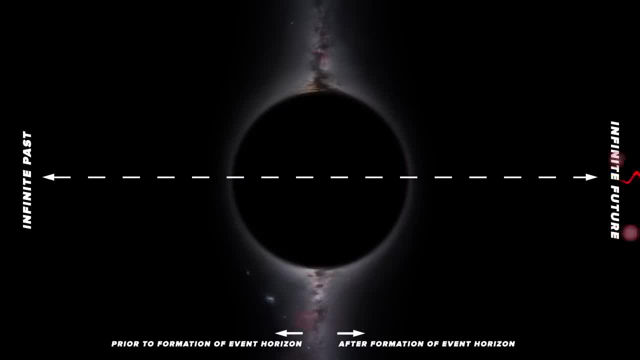 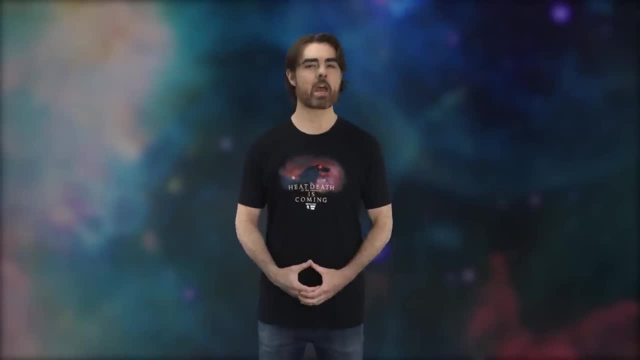 The vacuum should look like a vacuum. That's what we're looking for: A vacuum. This radiation is visible only to distant observers. Well, there is one exception: When you turn on your jet pack and hover a fixed distance above the horizon, then you do see particles. 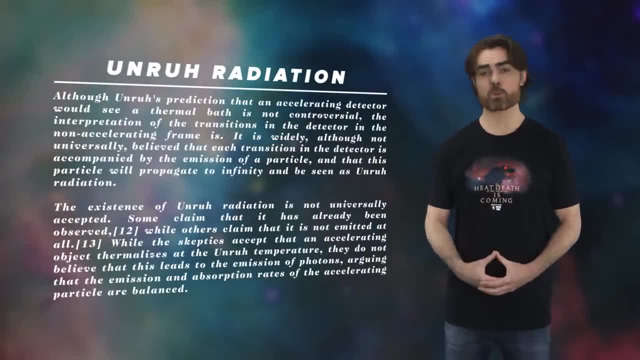 You see Unruh radiation. We'll look at its relationship to Hawking radiation in the future. By the way, Hawking radiation is mostly going to be photons and other massless particles. To produce particles with mass, the energy of the radiation. 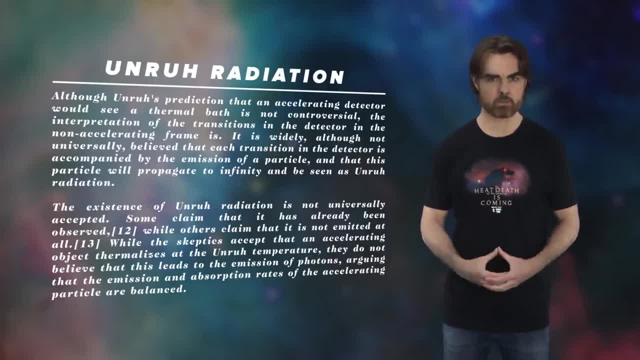 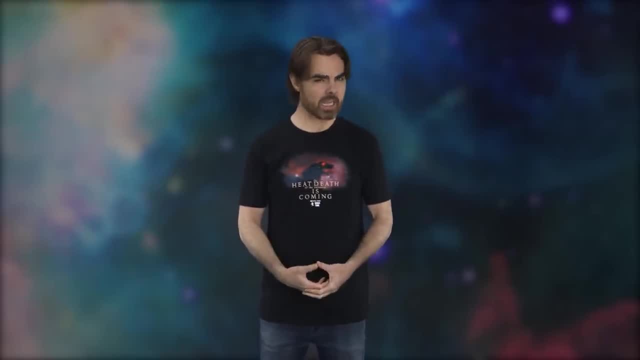 has to be high enough to cover the rest mass of the particle. So it's OK to interpret the narrative of Hawking's calculation as the splitting of entangled matter and antimatter pairs, even if it really is just a heuristic interpretation. It's the cause of the splitting that's hard to pin down. 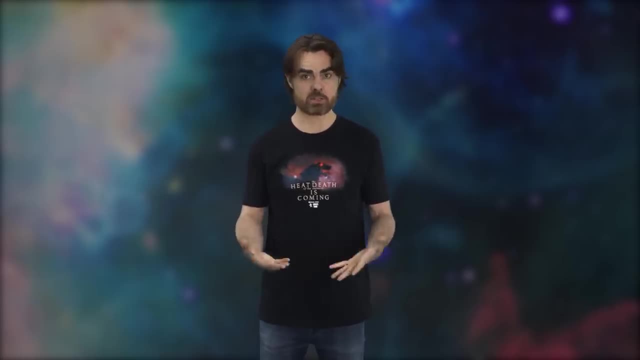 We can think about positive and negative frequency modes being mixed due to scattering, perhaps by the as yet undiscovered graviton. Other physicists have derived Hawking's result with very different seeming narratives, For example in 2001, Parikh and Wilczek. 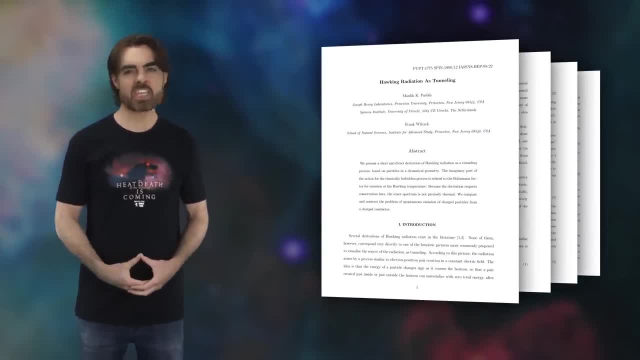 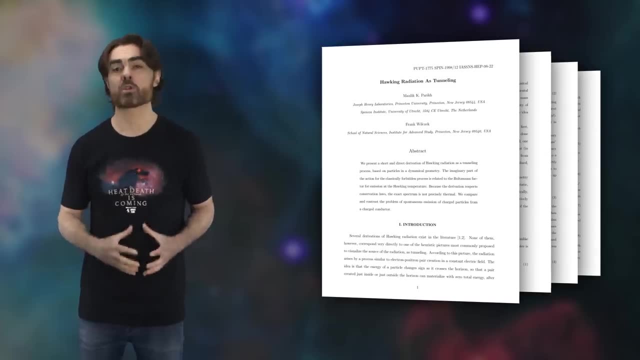 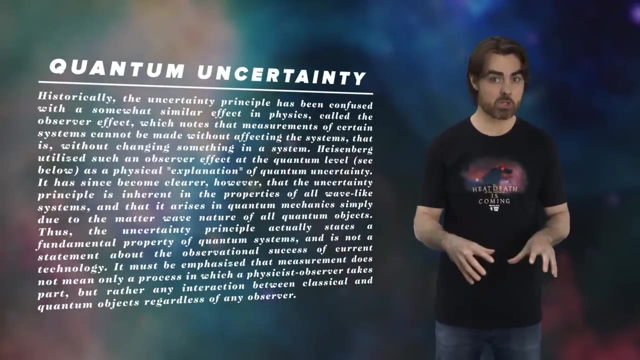 got the same thermal spectrum for Hawking radiation by thinking about particles escaping from beneath the event horizon through quantum tunneling. The common thread is quantum uncertainty. For example, uncertainty in position or momentum can lead to particle pairs that were once in the same location. 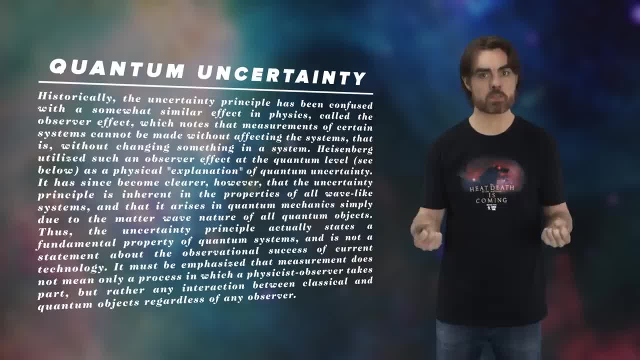 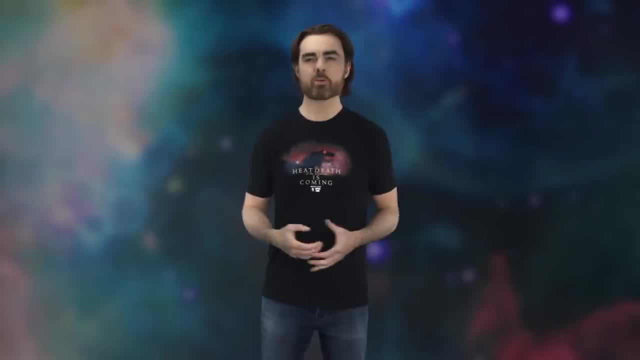 or modes that were once on the same world line becoming separated by the event horizon. Alternatively, uncertainty in energy can lead to particle creation. Whichever way you interpret it, it's hard to avoid the conclusion that black holes emit particles. The fact that different derivations lead to exactly